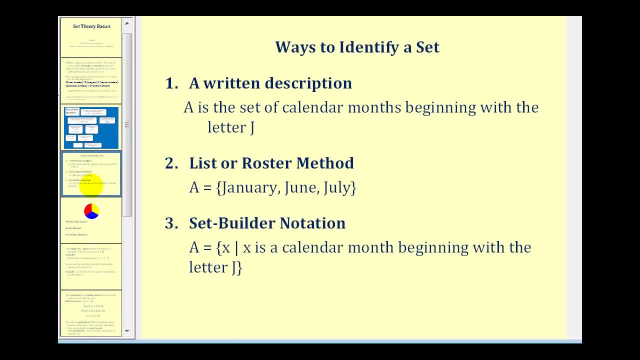 different ways of identifying a set. The first way is a written description. We could state that set A is the set of calendar months beginning with the letter J. We could also identify set A using the list or roster method, where we list the actual members of the set. 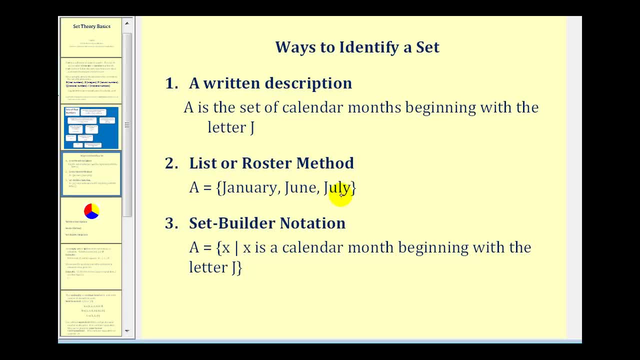 So set A is equal to January, June and July, And we could also use something called set builder notation. Set A is the set of all elements X, such that X is a calendar month beginning with the letter J. All these represent the same set. 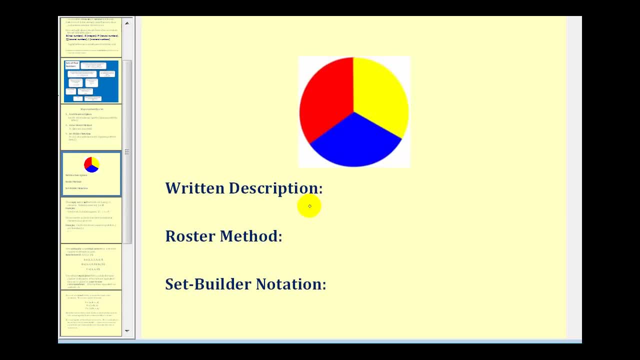 So describe the set of these three colors. The written description could be: B is the set of primary colors. Or, using the roster method, we could say that B is equal to the set, where the colors would be red, blue and yellow. Or using the set builder notation. 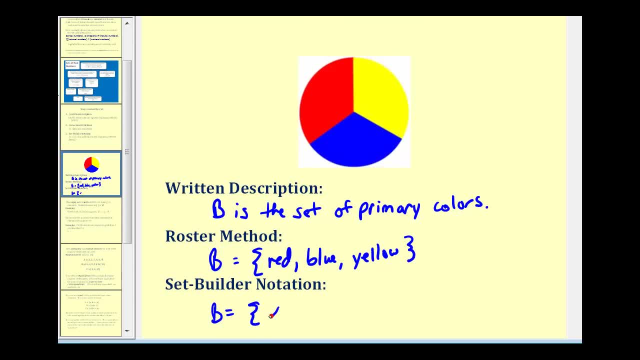 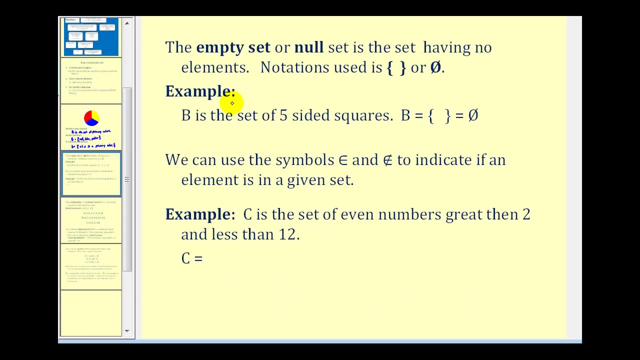 set B would be equal to the set of X, such that X is a primary color. There's also a special set called the empty set or null set. This is a set having no elements at all. The notation used for and empty set would be either of these two notations: 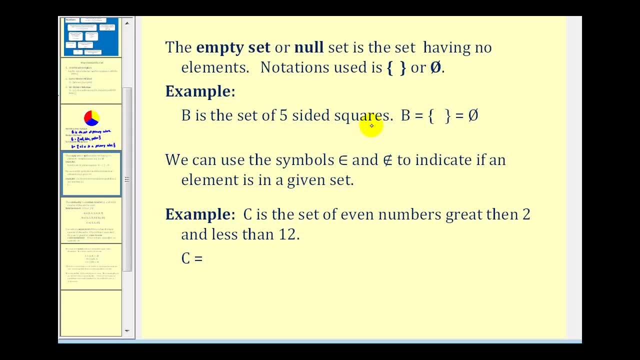 For example, if B is the set of five sided squares, since there aren't any five sided squares, B would be the null set or empty set, as identified here. We can also use these two symbols here in the set builder, here to indicate if an element is a member of a given set. 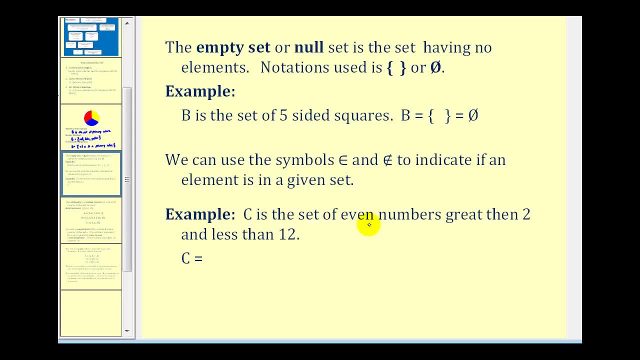 So, for example, if we have set, C is the set of even numbers greater than two and less than 12, let's first identify this set using the roster method. So we can't include two because two is not greater than two, So we'd have four, six, eight, 10.. 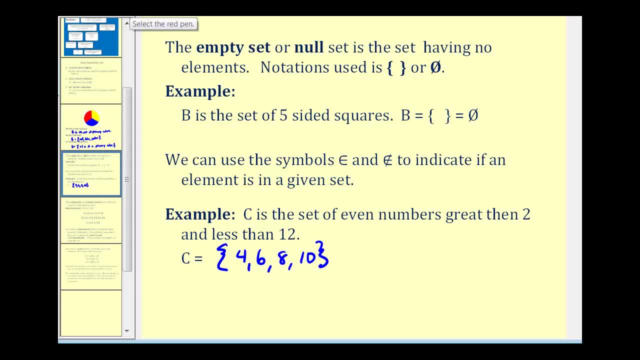 And we would also not include 12, because 12 is not less than 12.. So this is our set. So we could say that four is an element of set C, six is an element of set C, eight is an element of set C, and so is 10.. 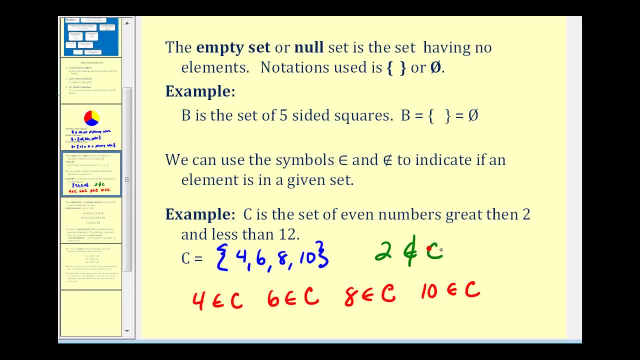 And we could also say that two is not an element of set C and 12 is not an element of set C, And of course there are many others. Now let's talk about cardinality, The cardinality or cardinal number of the set. 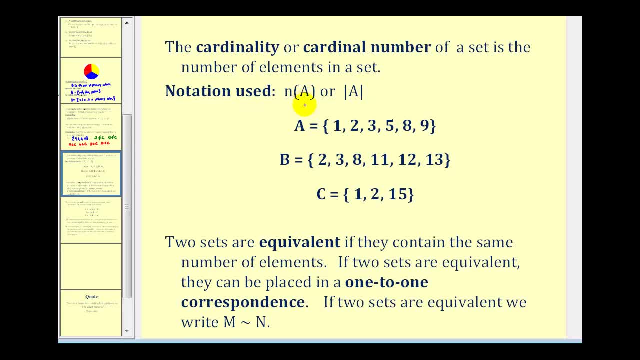 is the number of elements in a set And we normally use these two notations to represent the cardinality of a set. And since set notation does not repeat elements, we just have to count the number of elements in each set to identify the cardinality of the set. 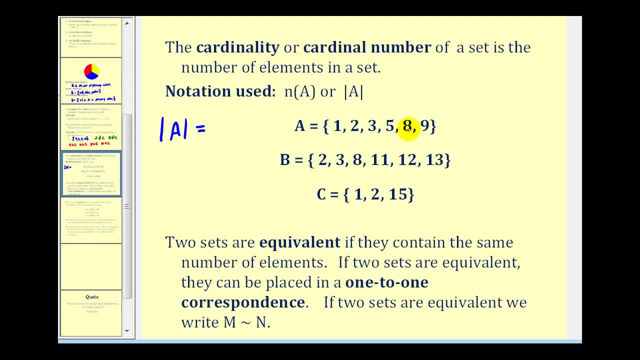 So the cardinality of set A would just be one, two, three, four, five, six. because there are six elements in the set, The cardinality of set B would be one, two, three, four, five, six as well. 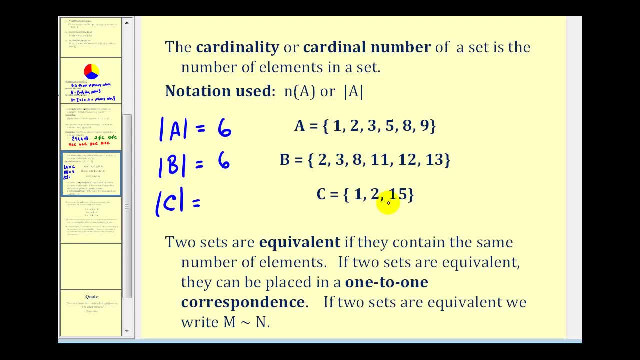 And the cardinality of set C would be three. Now, two sets are equivalent if they contain the same number of elements. If two sets are equivalent, they can be placed in a one-to-one correspondence. So if two sets are equivalent, we write their equivalent using this notation here: 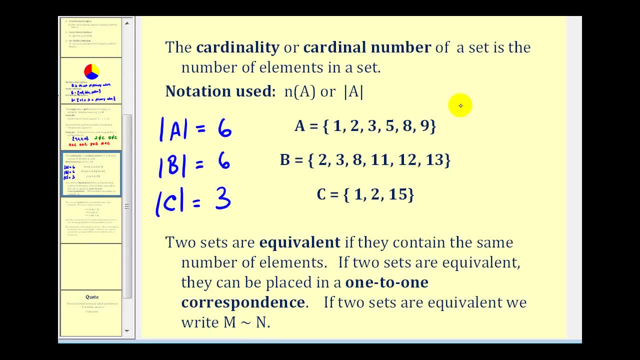 So looking at these two sets here, we could say that set A is equivalent to set B because they have the same cardinality or the same number of elements. Now we have to be careful about this word equivalent. Often in math it's used when things are equal. 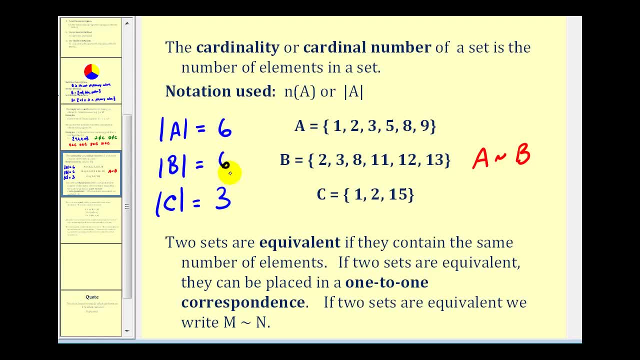 but obviously these sets are not equal. they just have the same number of elements. Now this idea of a one-to-one correspondence just means that for every one element in set A, we could match it with one element in set B, So we could match one with two. 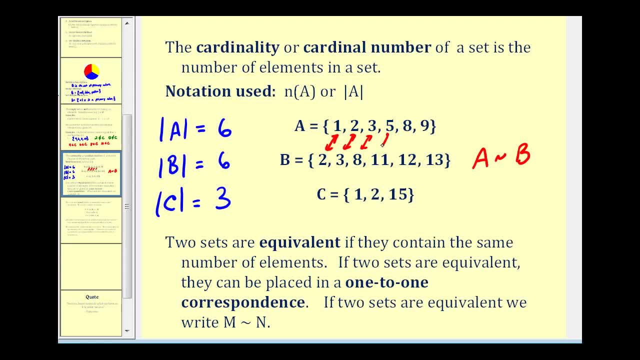 two with three and two with four, two with three, three with eight, five with eleven, eight with twelve and nine with thirteen, illustrating the one-to-one correspondence. The last topic we'll talk about in this video is when two sets are equal. 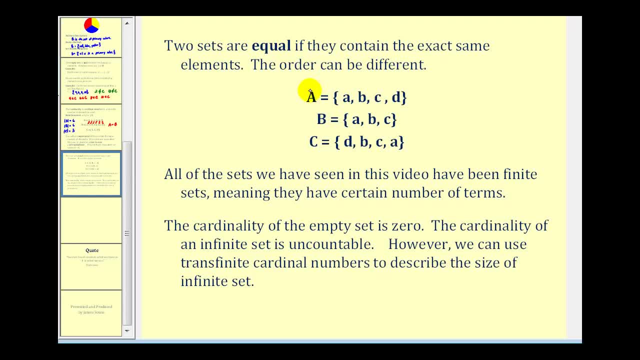 Two sets are equal if they contain the exact same elements that may or may not be in the same order. So looking at these three sets here, notice that set A and set C have the same cardinality, meaning they have the same number of elements, and they also have the exact